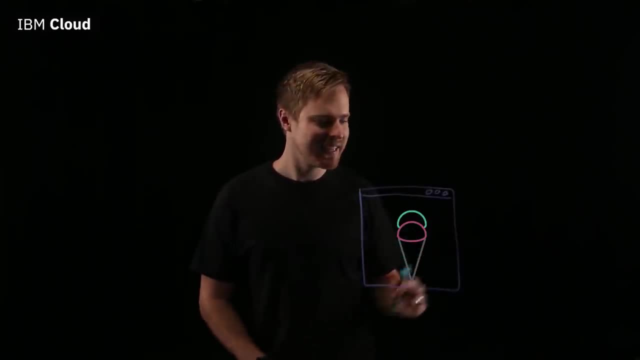 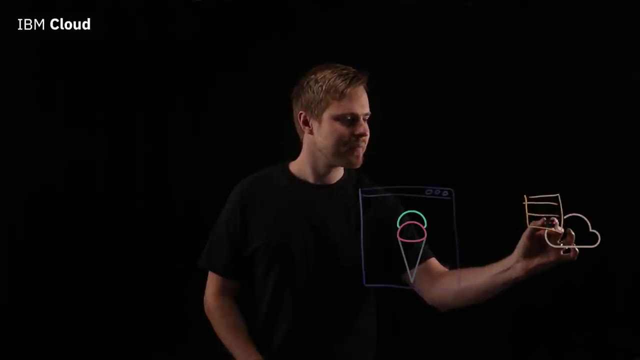 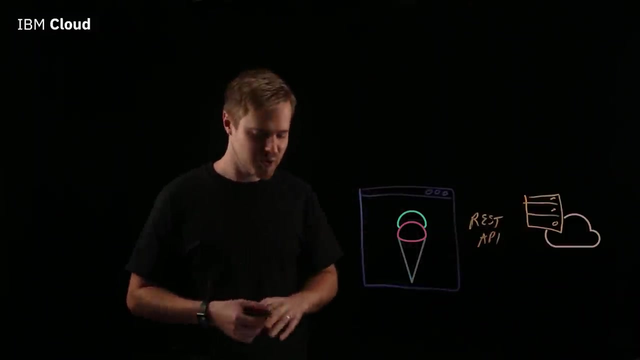 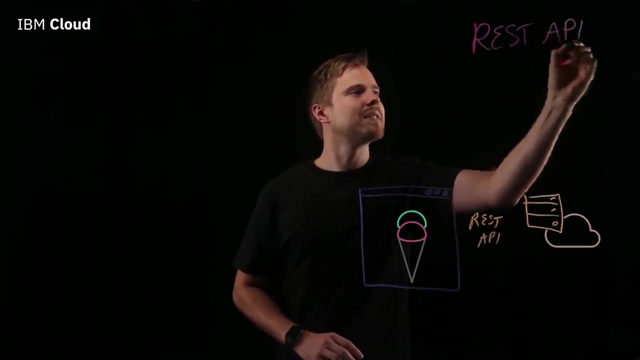 How do you do this? Well, with a REST API. You have your web app or web page communicate with a cloud-based server via a REST API- Great, So let's jump into what exactly a REST API is. Starting out with. what does REST stand for? 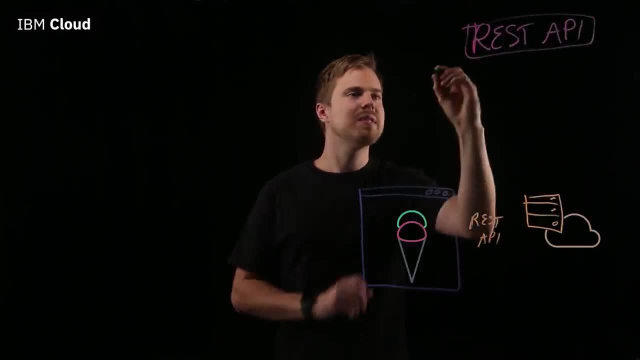 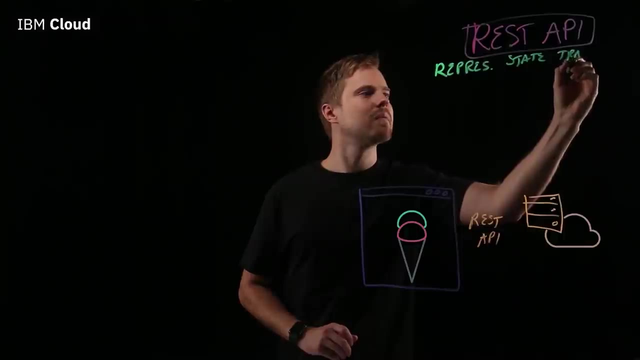 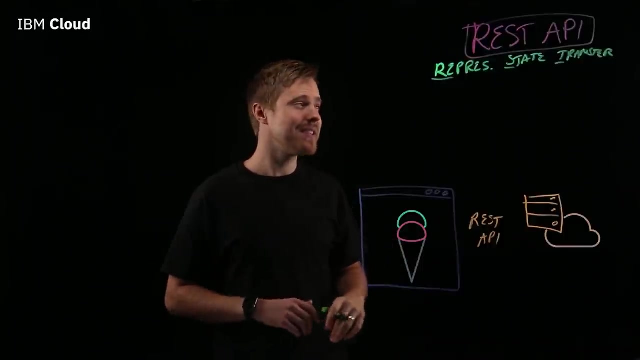 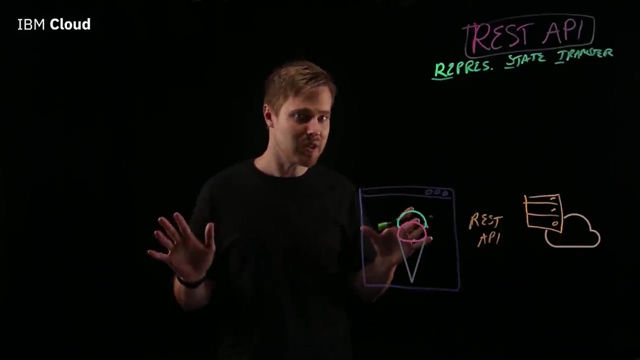 Right. so REST stands for Representational State Transfer, So it's REST, Right. those words might not mean a whole lot to you, but basically it's a standardized software architecture style of a specific type of API that's industry known and used. 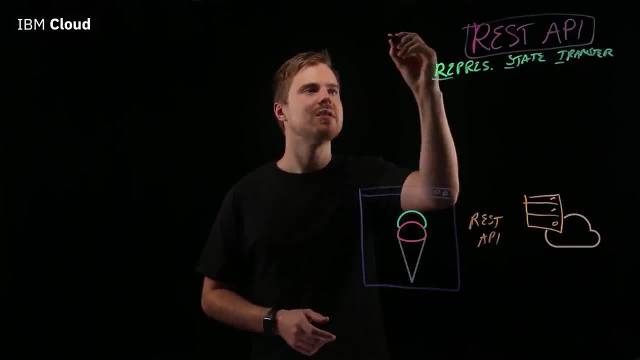 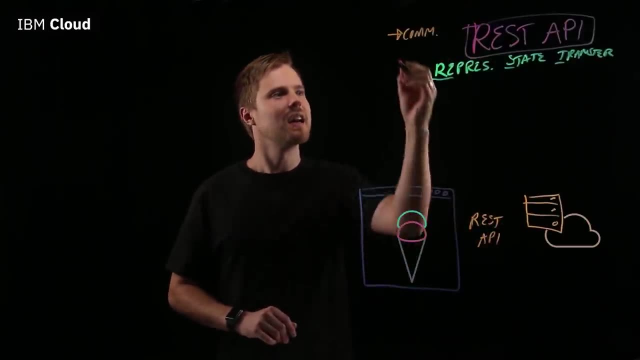 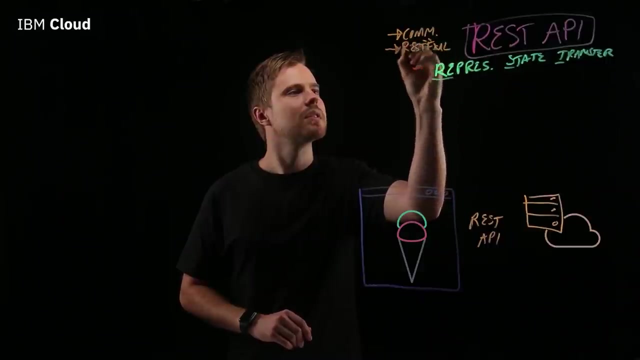 So the first thing that you should really know about REST APIs is: they're all about communication, So client with server and vice versa. that's how they talk. And also you may have heard the term RESTful, So RESTful web service, right. 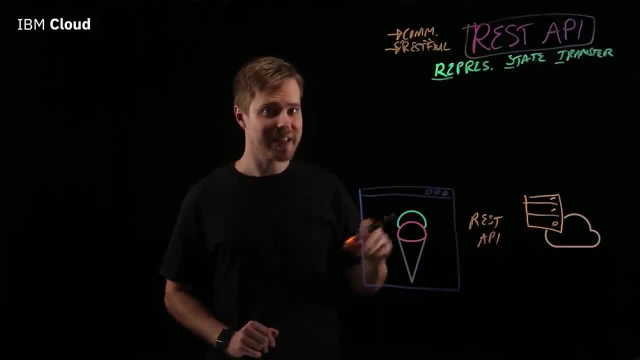 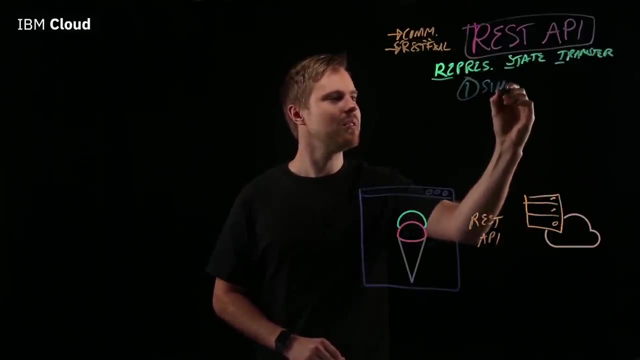 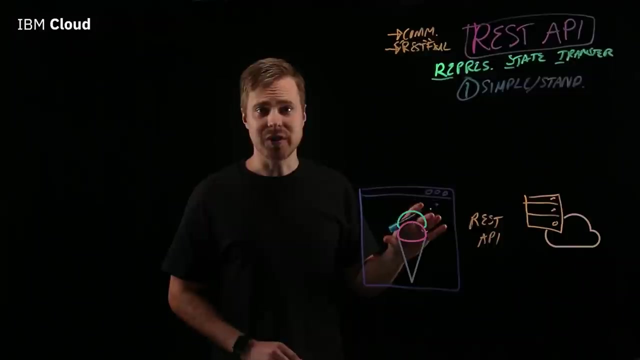 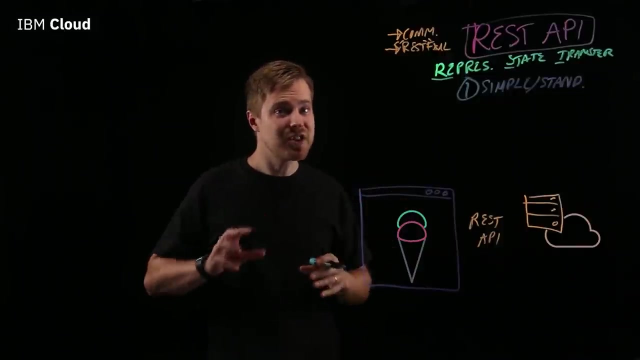 That's a service that uses REST APIs to communicate. So what are some of the benefits of REST APIs? First of all, they're simple and standardized. You don't have to worry about how to format your data or how to format your request each time. 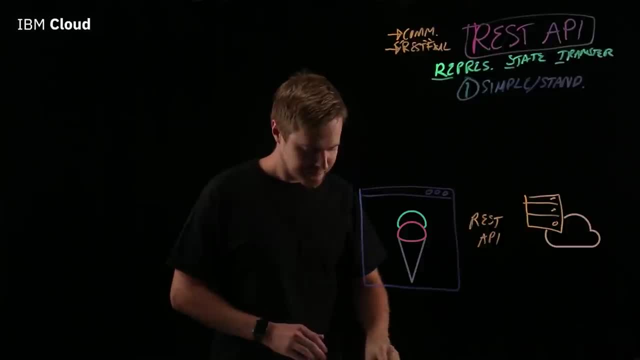 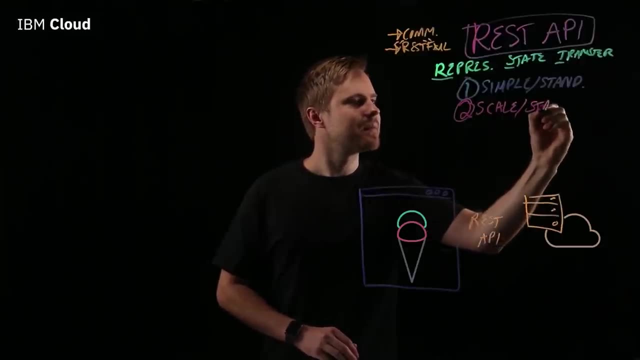 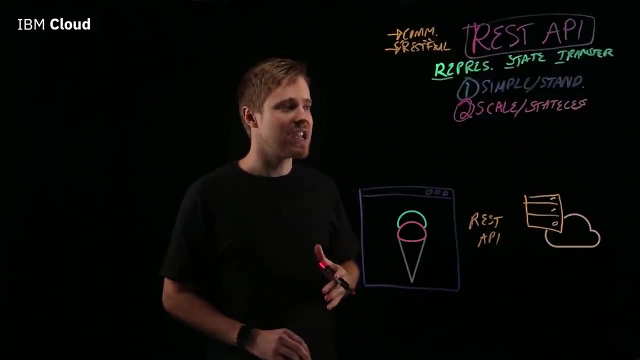 It's all standardized and industry used. Second of all, REST APIs are scalable and stateless, So as your service grows in complexity, you can easily make modifications, And just the fact that they're stateless means you don't have to worry about. 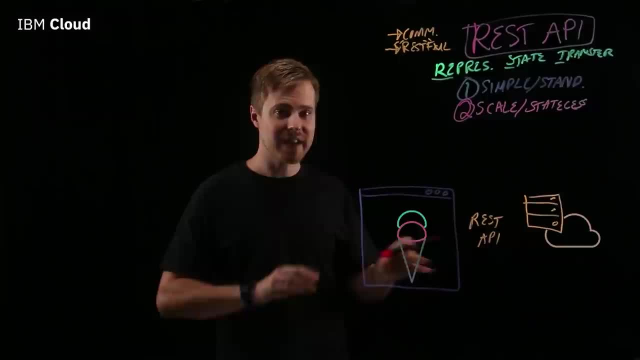 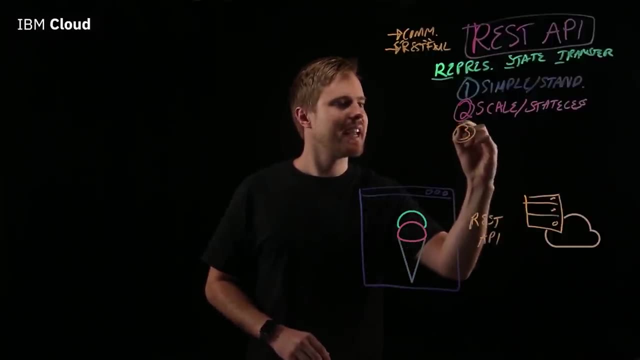 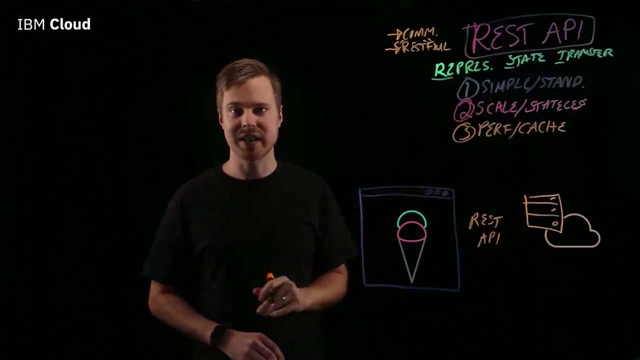 what data is in which state and keep track of that across client and server. It's truly stateless, Great. And then, finally, they have high performance, in large part due to the fact that they support caching. So that's all good stuff. 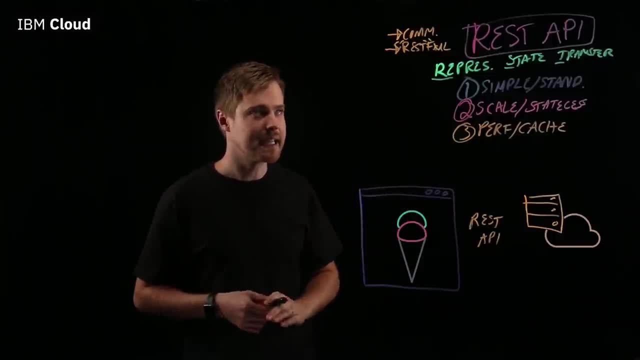 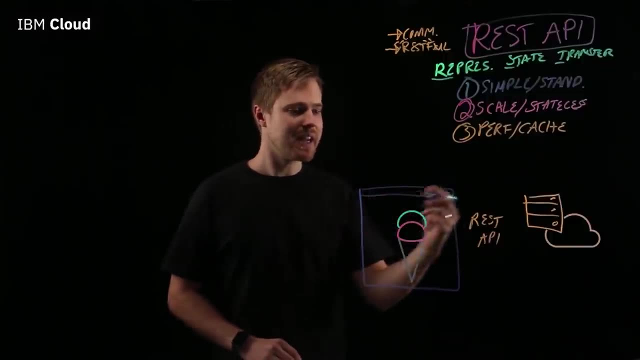 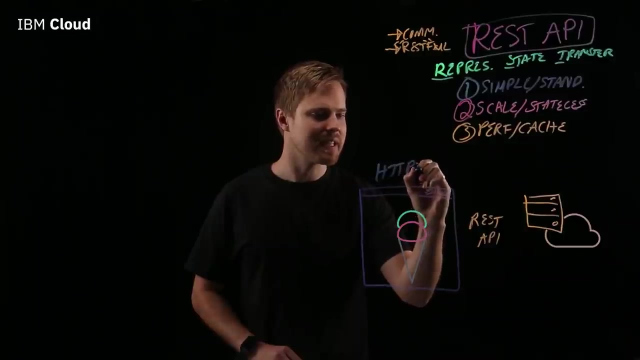 As your service gets more complex, the performance stays very high. Great, So let's go back to our example. So, for the ice cream shop, what would the REST API look like? right? So you have an endpoint which might look something like this: 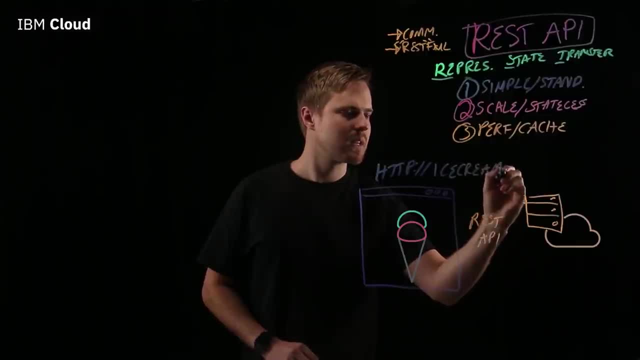 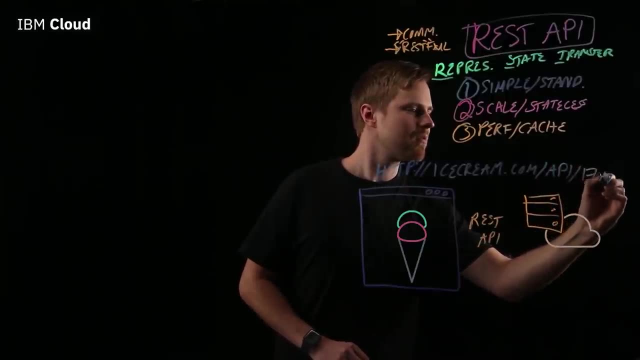 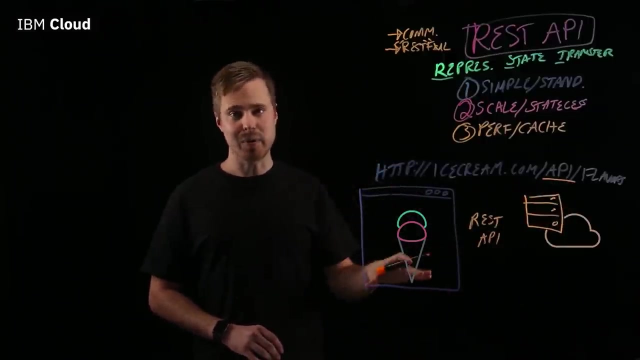 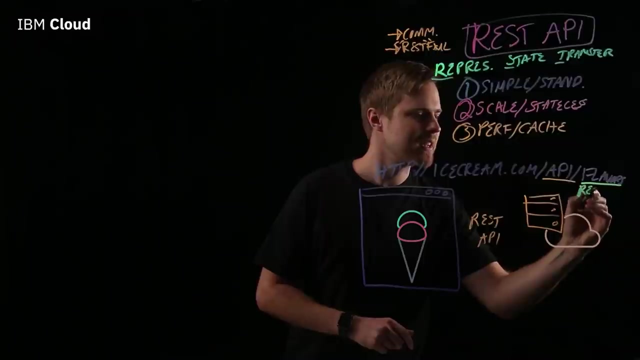 icecreamcom: slash API, slash flavors, right? So let's break that apart a bit. So API, this just signifies that this is the API portion of the endpoint, right? Pretty straightforward. there, Flavors is actually what's known as a resource. 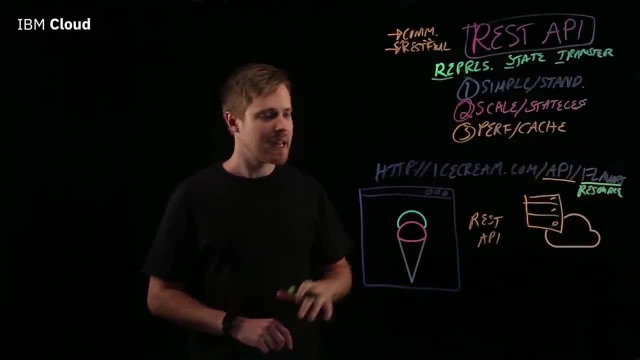 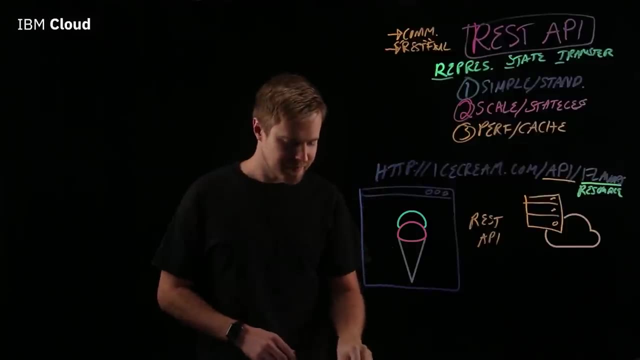 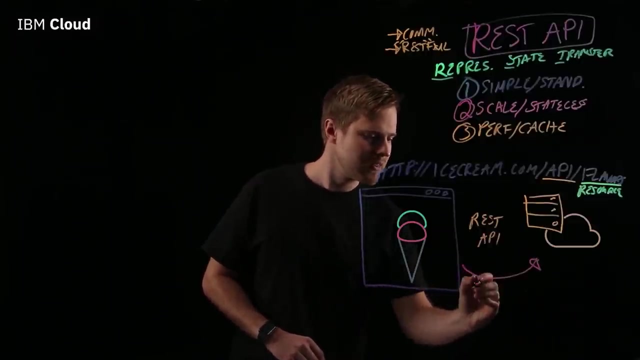 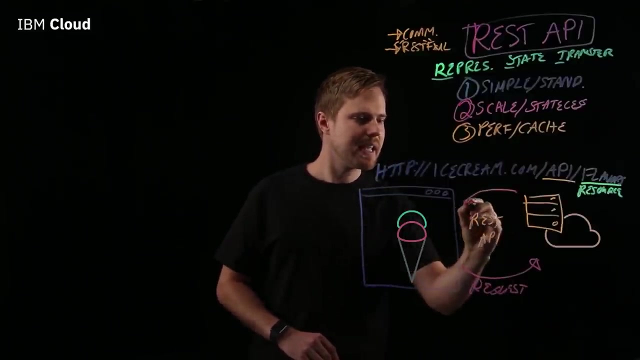 So this signifies that we're working with the flavors resource in this REST API- Great. So in our example, the main building blocks or parts of the REST API are the request that is sent from the client to the server and the response that is received back. 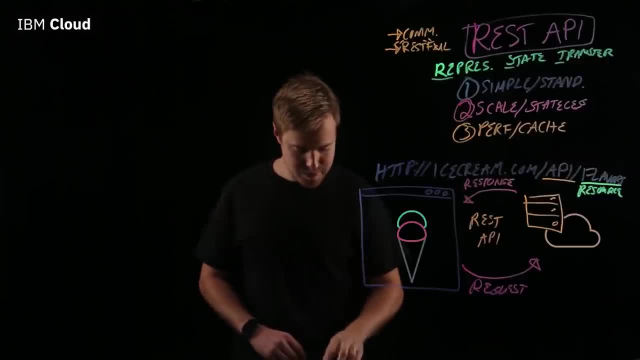 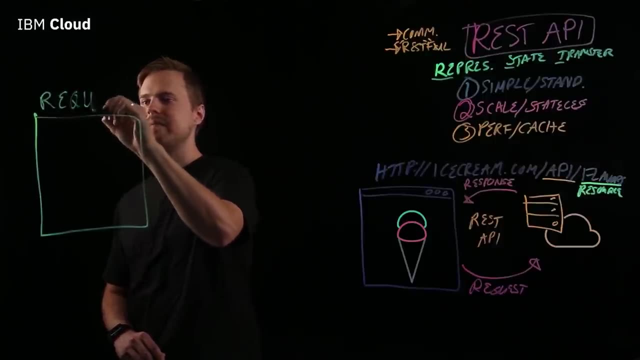 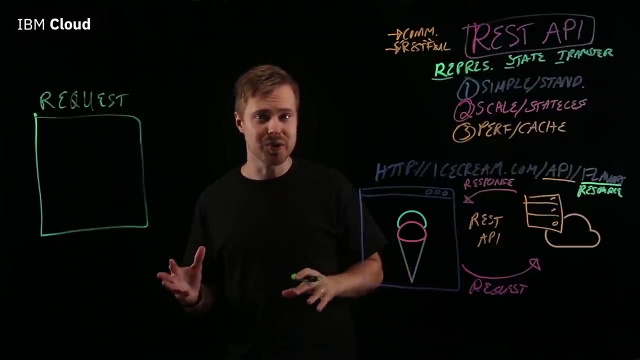 from the server, right? So let's break those apart a little bit Over here. let's put a big old box for request And what are the type of things that you might want to do with a REST API? What actions or verbs would you want to make? 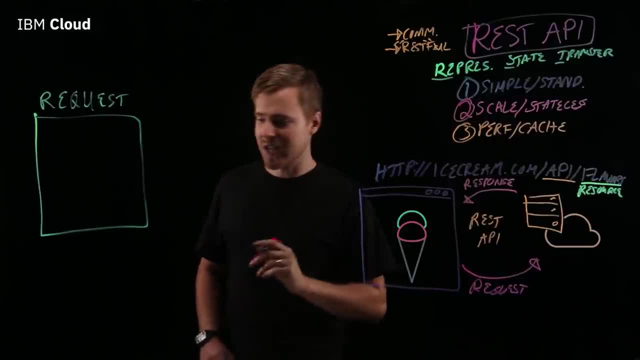 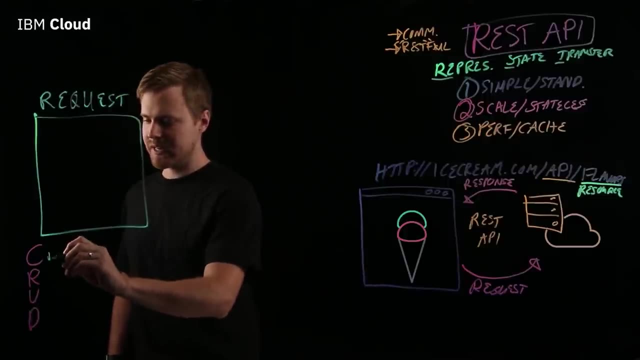 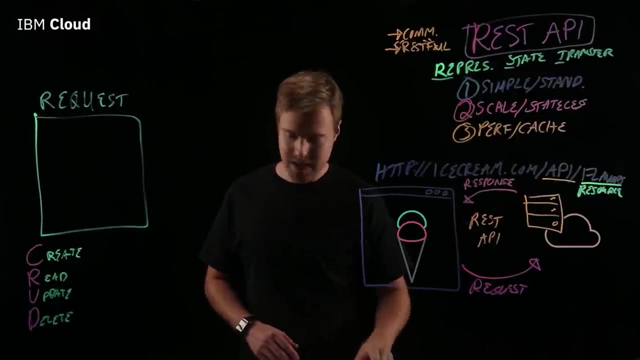 when you're working with one. You may have heard of CRUD. What does CRUD stand for? So CRUD is create, read, update and delete. These are some of the main things that you might want to do when you're communicating with your client and server. 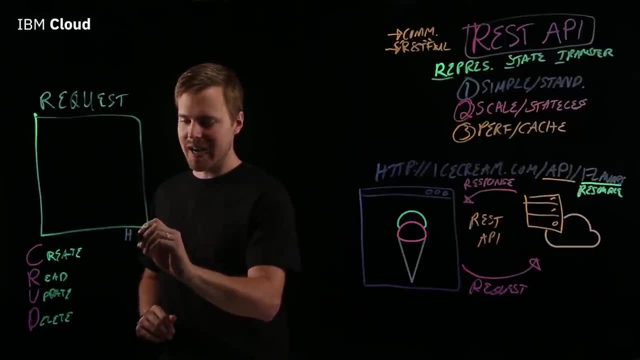 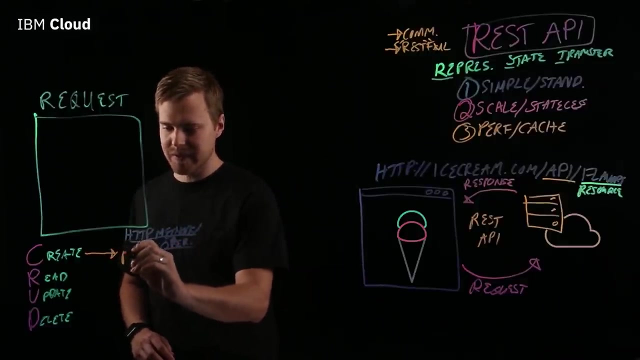 On a REST API. the equivalent of those are actually HTTP methods or operations. Right? so what's the equivalent of create in a HTTP method? Well, it's post. And how about read? So read is actually called, get, Update or replace is put. 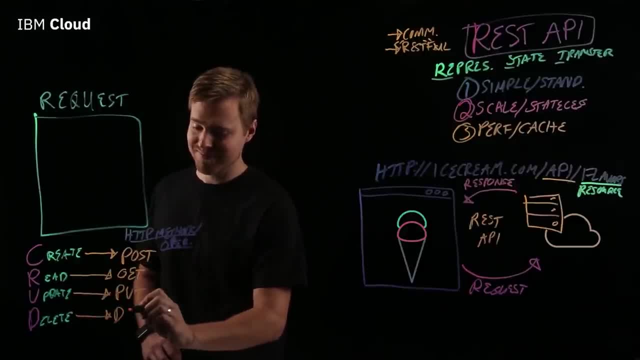 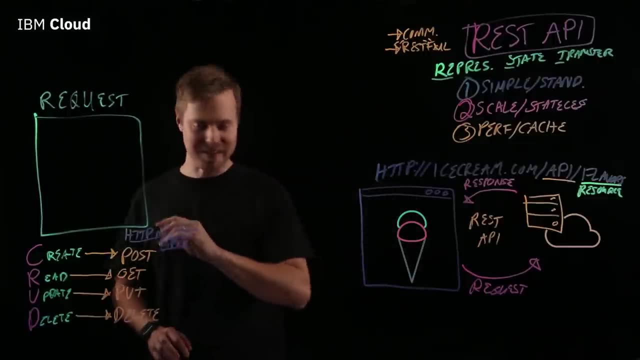 And delete. guess what it is? Delete- Not too creative there. So how about a request itself? What are some of the pieces of it? So, first of all, you might have an operation. That's kind of what we just talked about here. 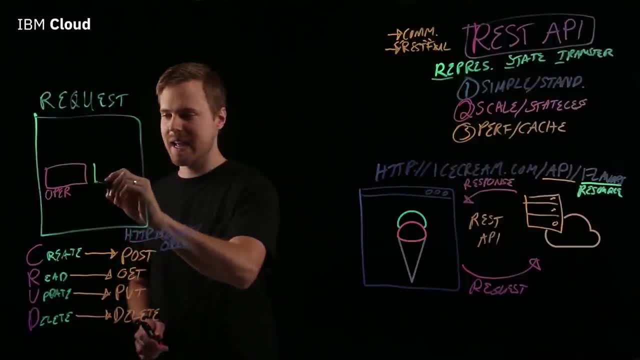 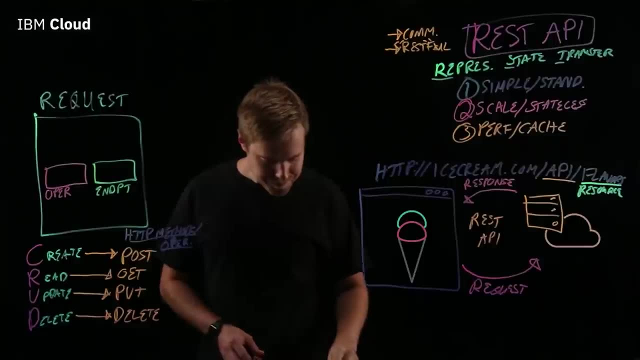 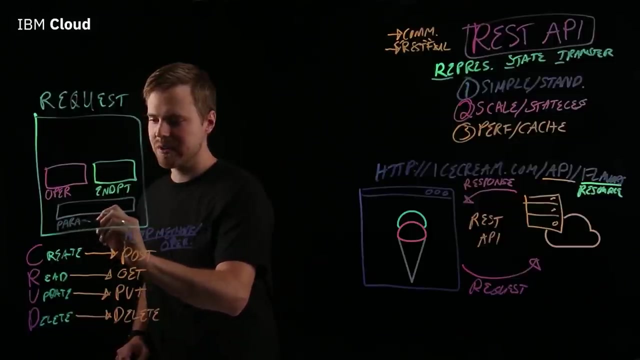 with the HTTP methods. You might have an endpoint, which is what we just talked about over here. This is your REST API endpoint. And then you might also have parameters or body, which is some data that you might send in the request, And we'll see some examples in a moment. 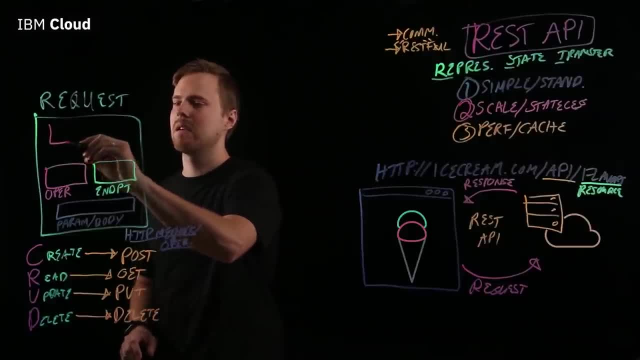 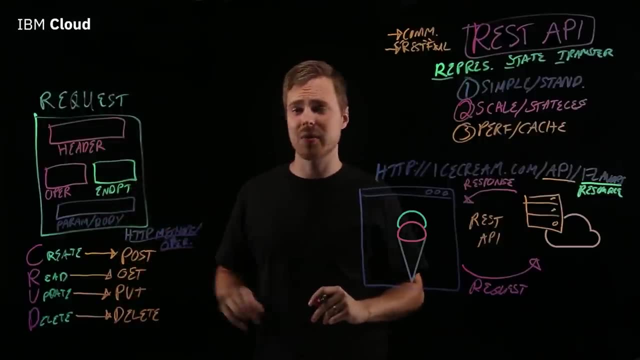 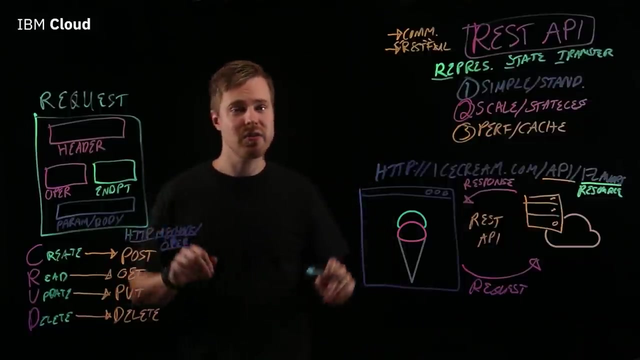 And finally are the headers. So this is a special part of an API REST, API request, which might have things like an API key or some authentication data- Great, And then in return from the server, you'll receive a response, right. 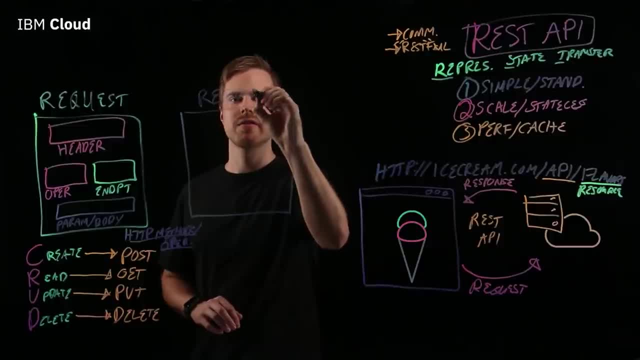 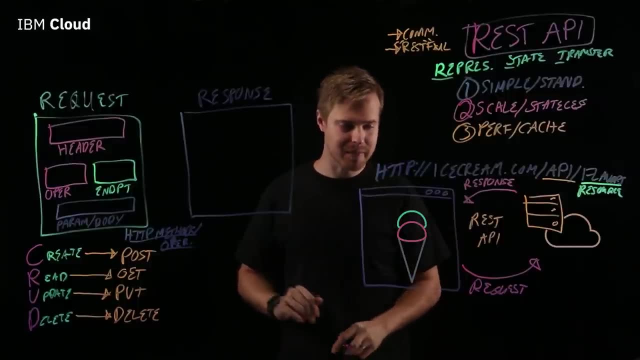 So we'll put a nice box here for response, And this is typically in the form of JSON data. Great, So let's jump into our example And let's look at a few different scenarios that might happen with your ice cream shop, right? 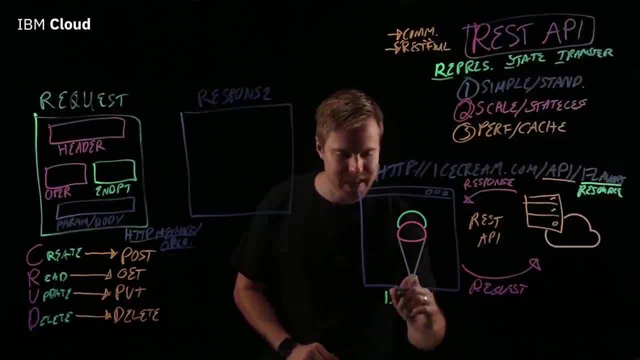 So, first of all, let's say that you want to display what's currently in stock, right? So we want to get the flavors that are in stock. So what does our REST API request look like? Well, you have a get as the operation. 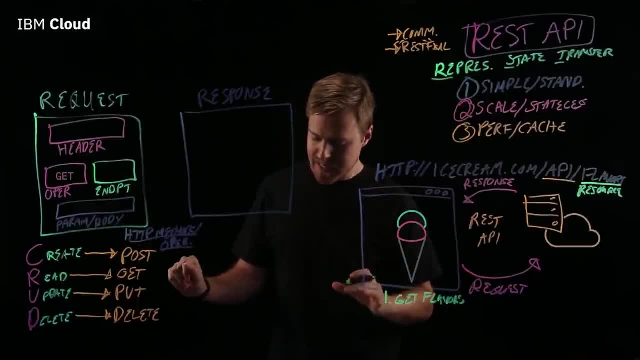 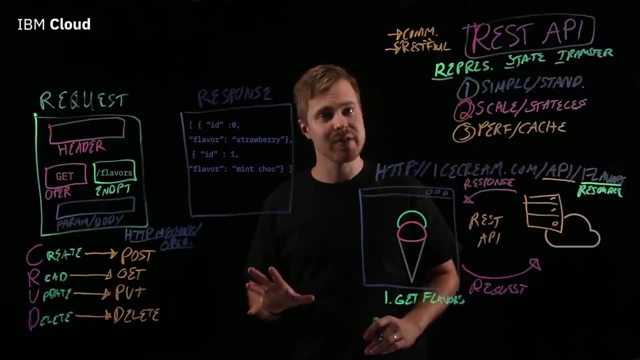 because you're actually wanting to get those flavors, And then the endpoint is: slash API, slash flavors, And in response you'll get an array of those flavors, flavor resources right. So we see strawberries in stock as well as mint chocolate- Yummy. 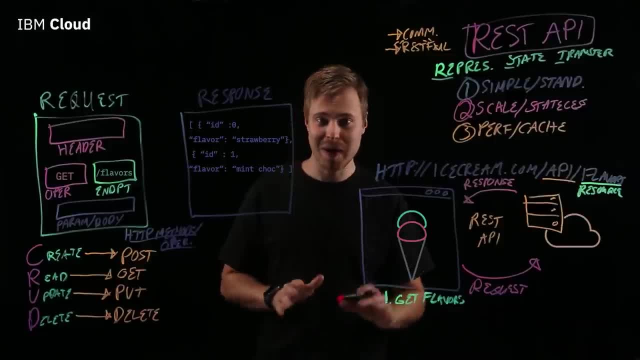 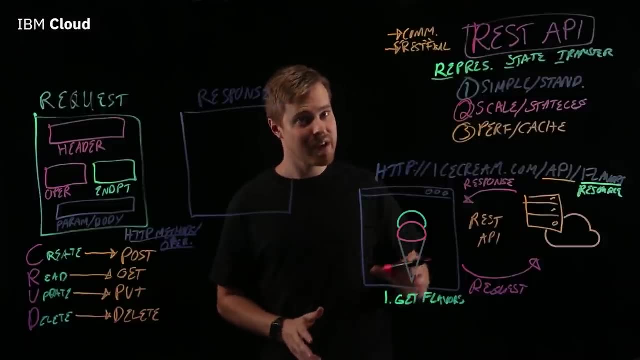 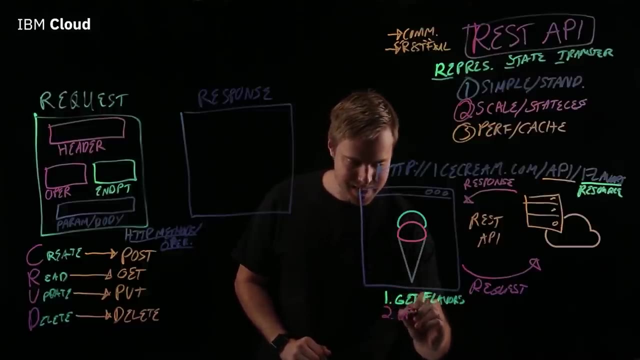 But then, uh-oh, Mint chocolate is so popular that it actually runs out for the day And the store is scrambling and they want to replace that flavor with another one. They choose chocolate, which is a great choice. So let's say they want to update. 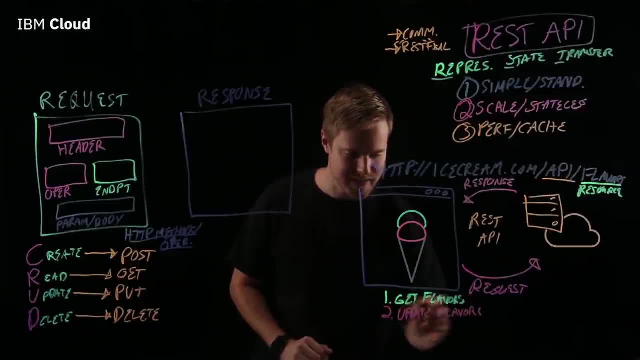 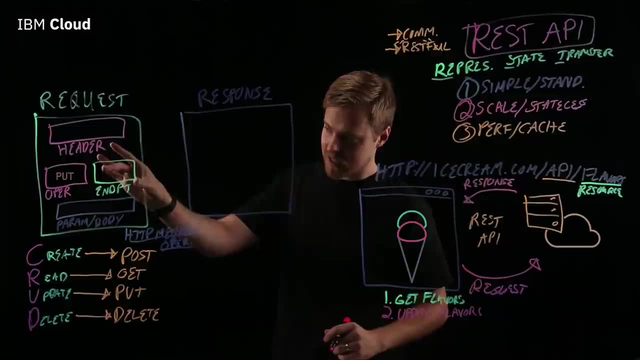 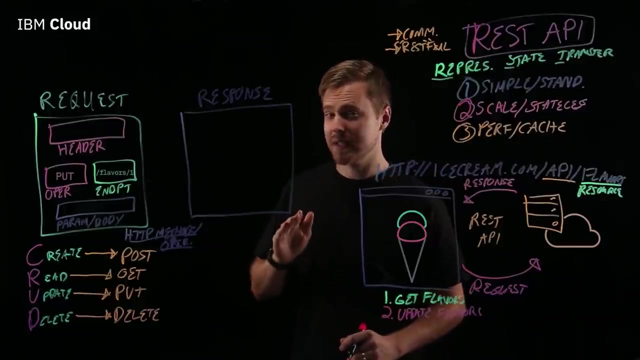 the flavors, right. So you want to update or replace that mint chocolate with just chocolate. So what does our request look like? It's a put operation So that updates or replaces. The endpoint is: slash API, slash flavors, slash one to indicate the ID of one you want to replace.